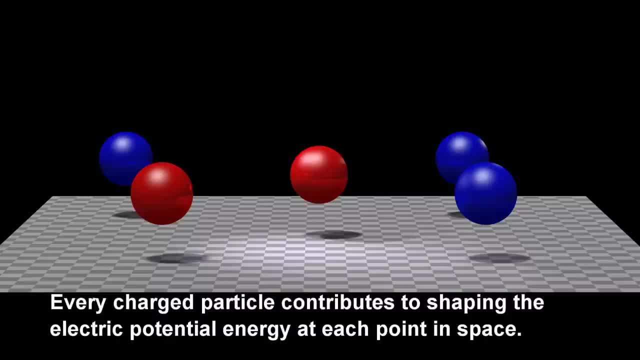 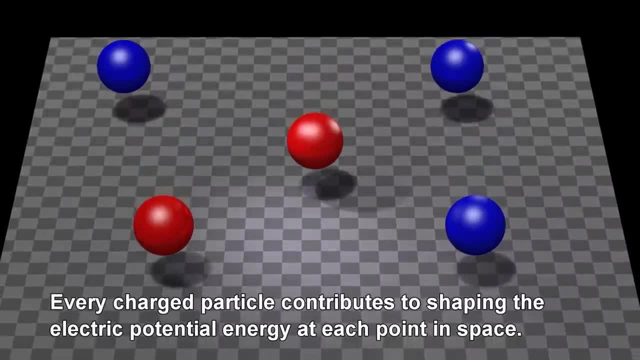 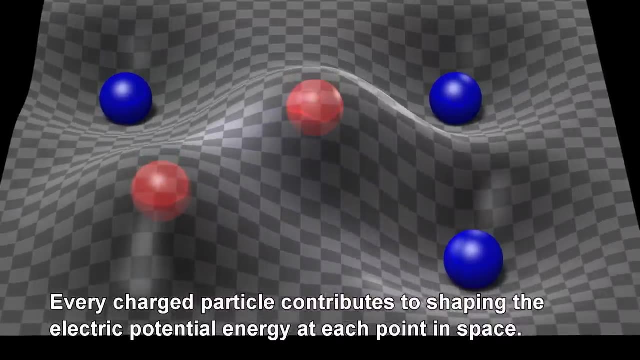 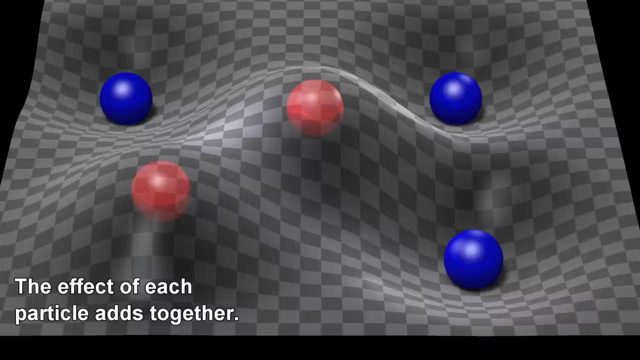 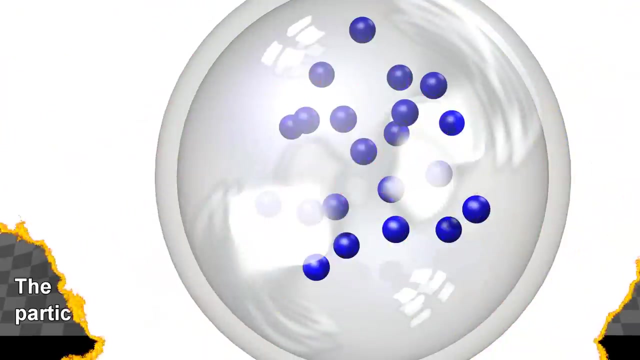 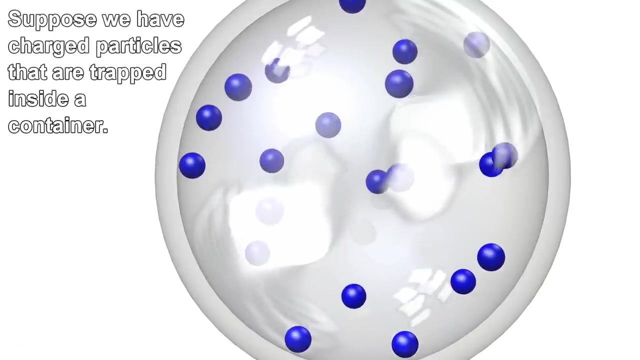 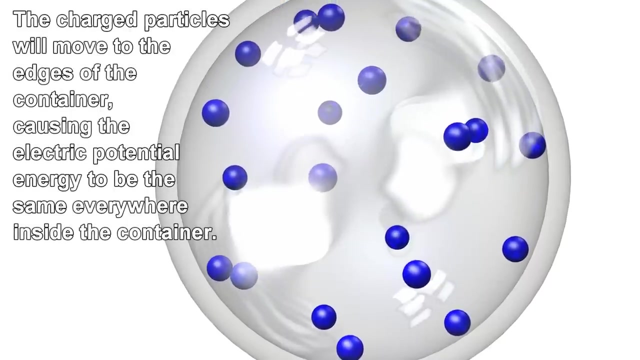 Every charged particle contributes to shaping the electric potential energy. at each point in space The effect of each particle adds together. Suppose we have charged particles that are trapped inside a container. The charged particles will move to the edges of the container, causing the electric potential energy to be the same everywhere inside the container. 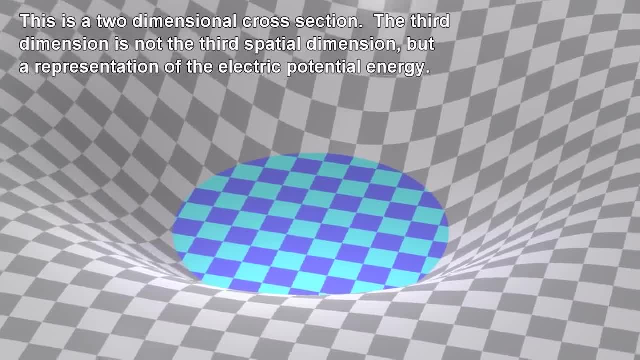 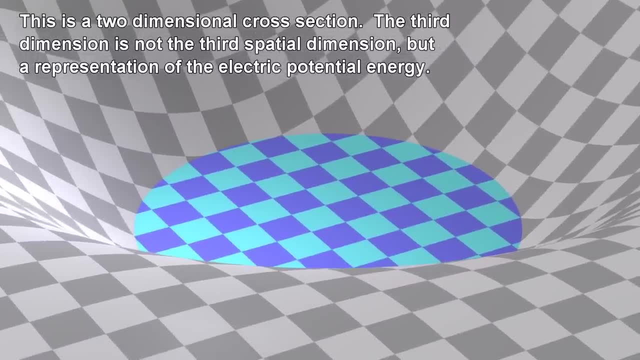 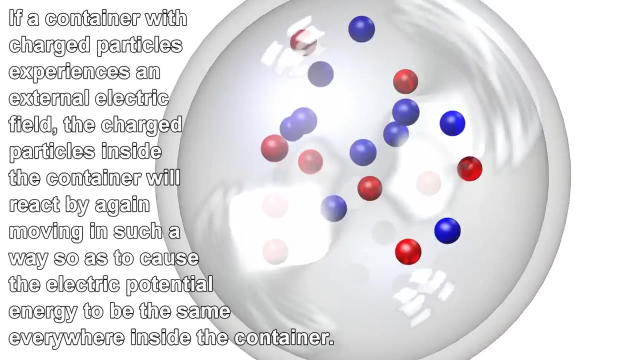 If we move the charged particles into a container, the electric potential will expand and the electrical field will react to gözelski, and thus Сейчас we are getting more and more charged particles and the electrical field is different. As for the effect of magnetic field on electronic elements is the same everywhere within the container. 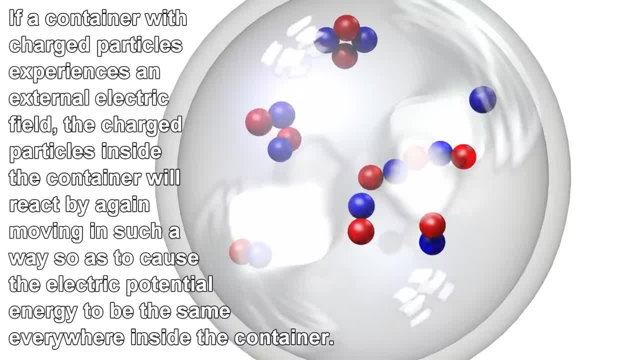 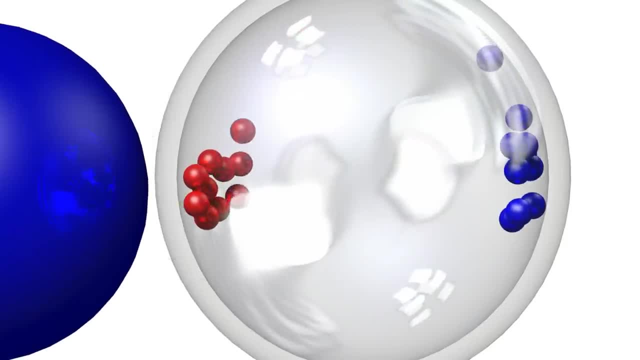 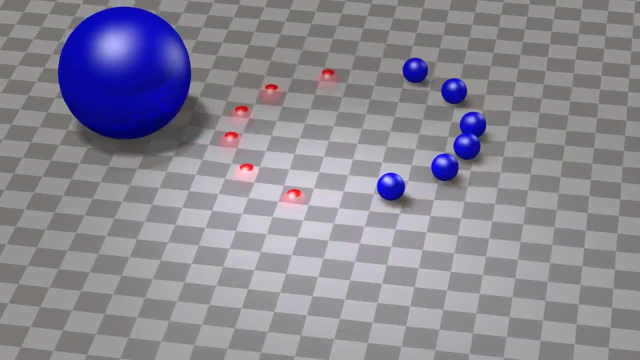 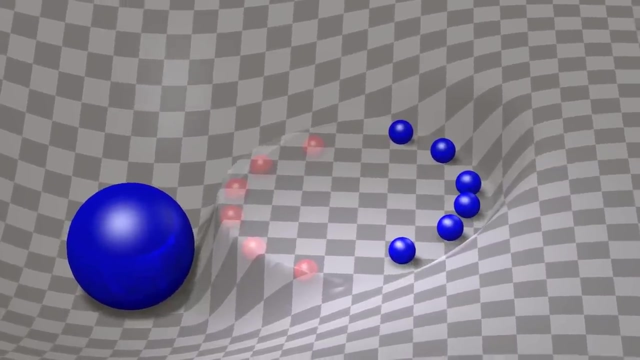 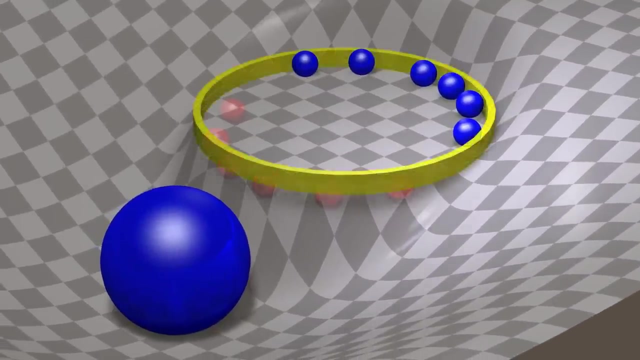 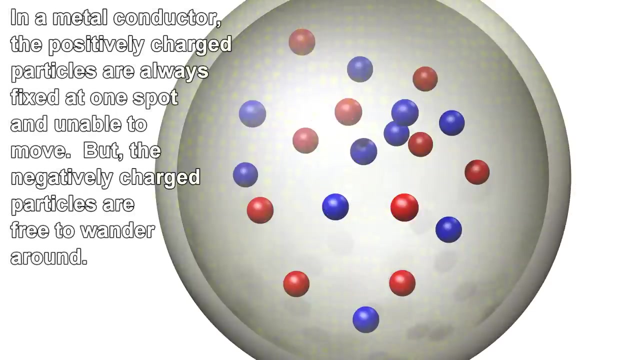 ımı the container. The charged particles inside the container will react by again moving in such a way so as to cause the electric potential energy to be the same everywhere inside the container. In a metal conductor, the positively charged particles are always fixed at one spot and unable to move, but the negatively charged particles are free. 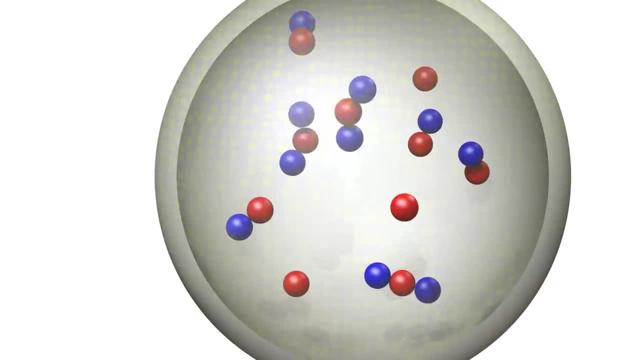 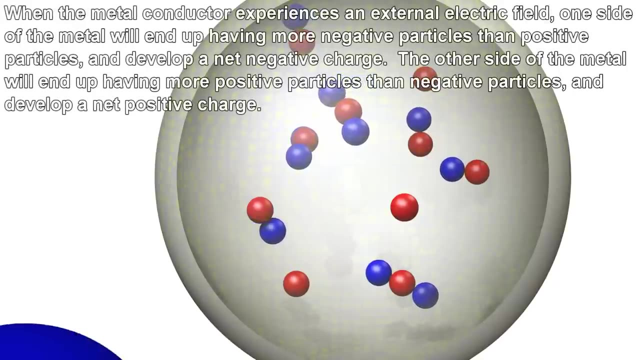 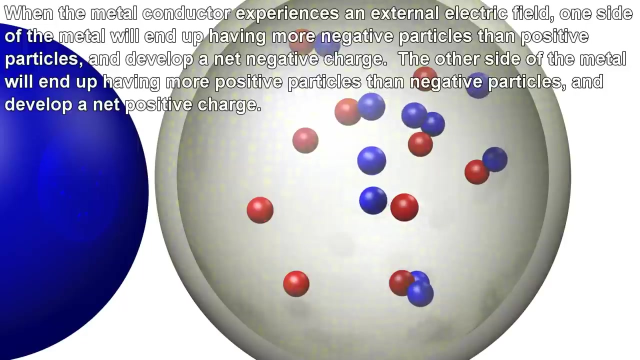 to wander around. When the metal conductor experiences an external electric field, one side of the metal will end up having more negative particles than positive particles and develop a net negative field. The other side of the metal will end up having more positive particles than. 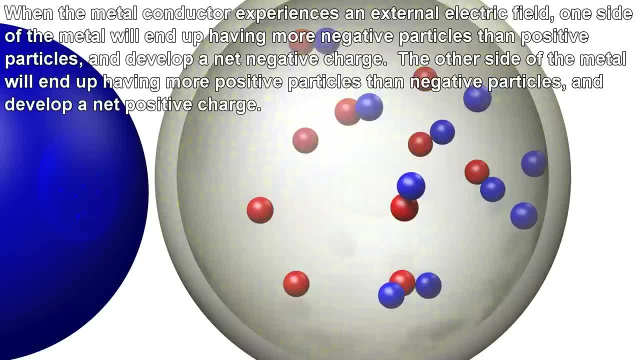 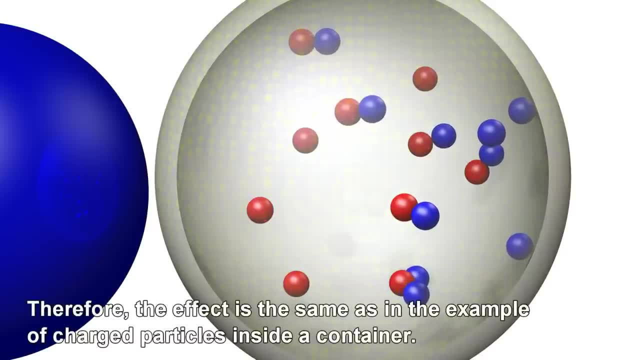 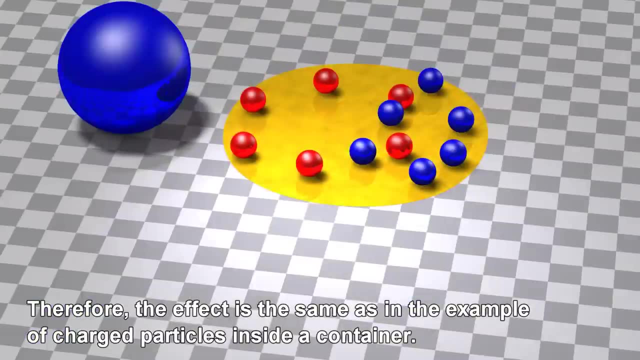 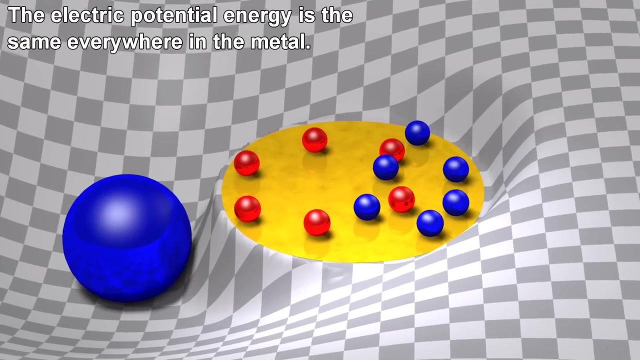 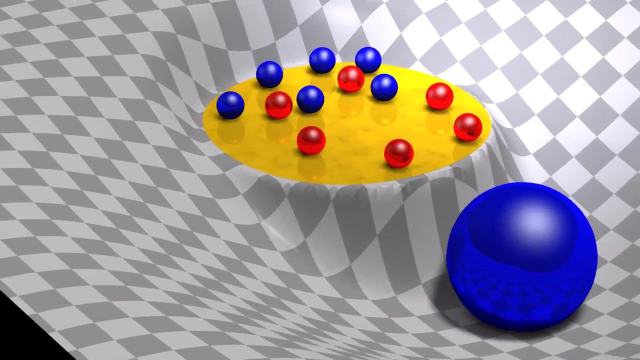 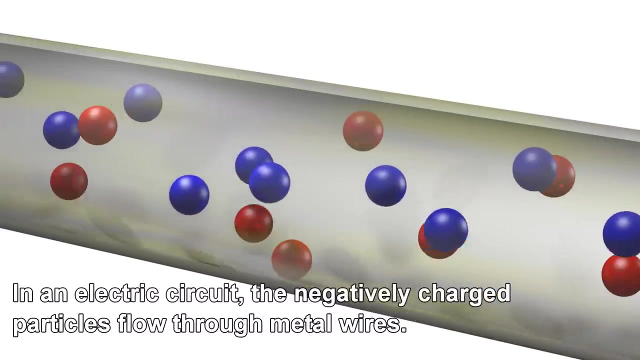 negative particles and develop a net positive charge. Therefore the effect is the same as in the example of charged particles inside a container. The electric potential energy is the same everywhere in the metal In an electric circuit. the negatively charged particles blow through metal. 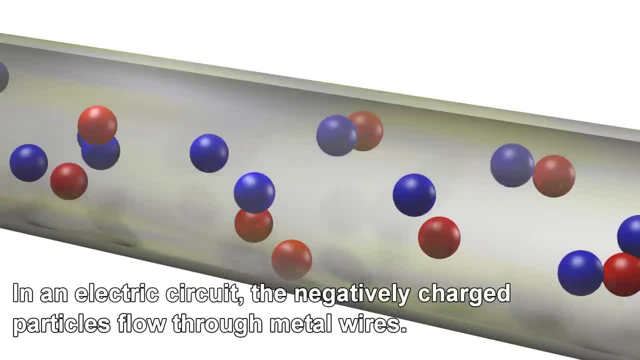 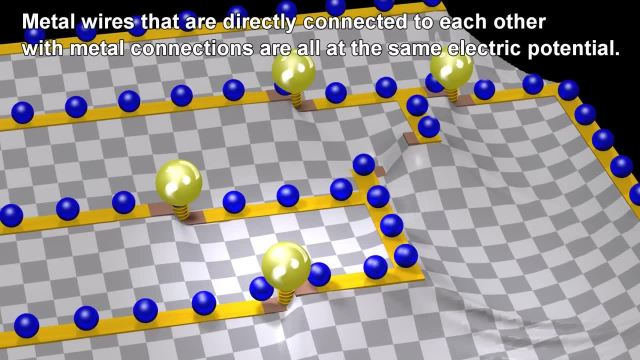 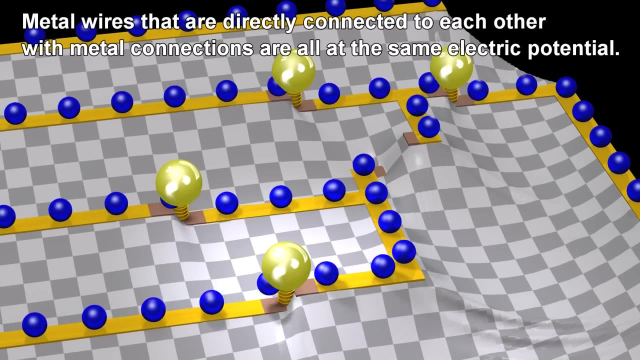 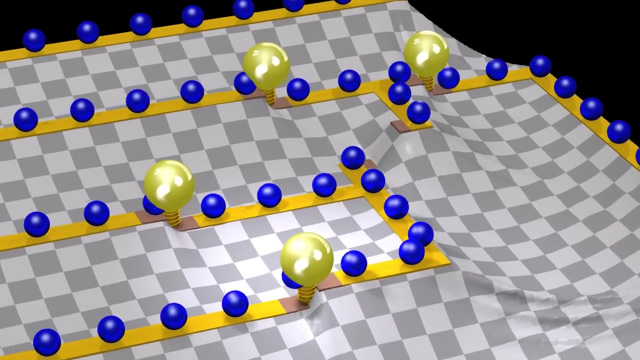 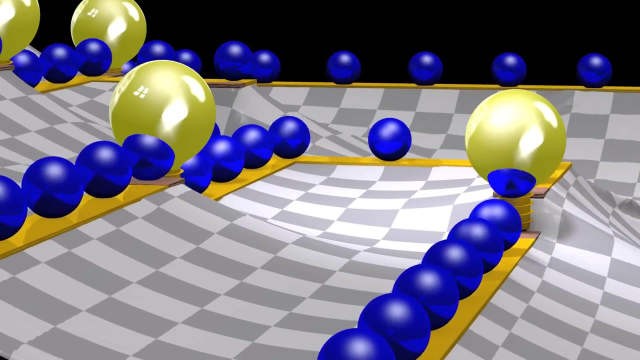 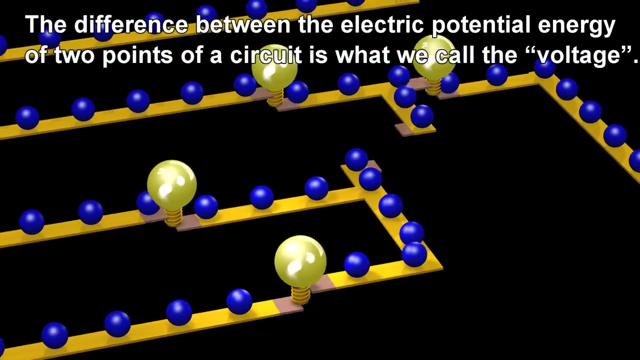 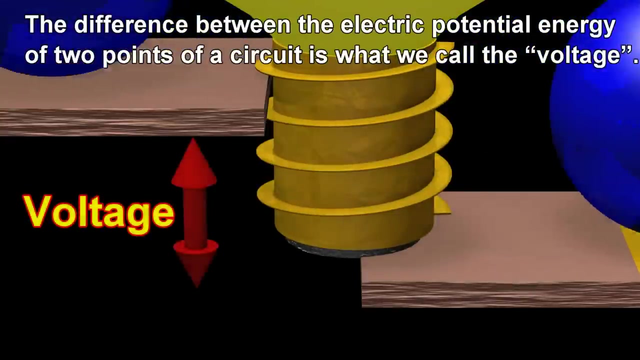 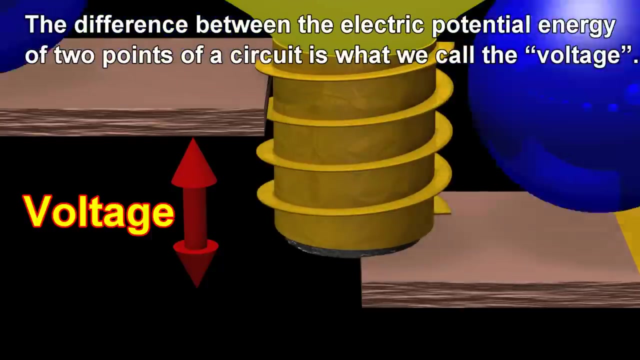 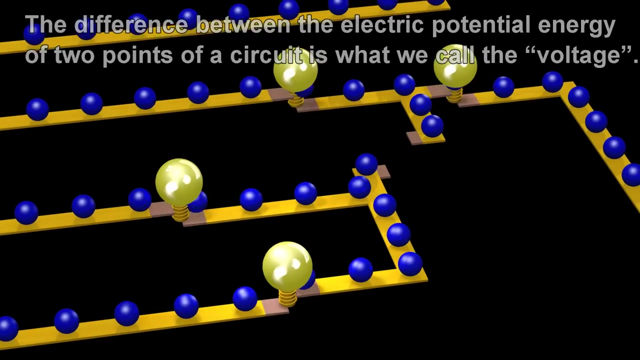 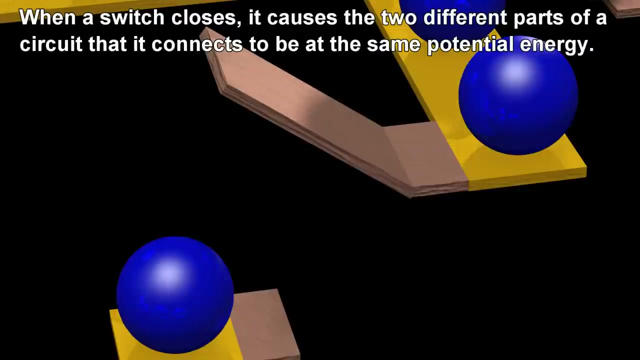 wires, Metal wires that are directly connected to each other with metal connections, are all at the same electric potential. This is the dark. The difference between the electric potential energy of two points of a circuit is what we call the voltage. When a switch closes, it causes the two different parts of a circuit that it connects to to. 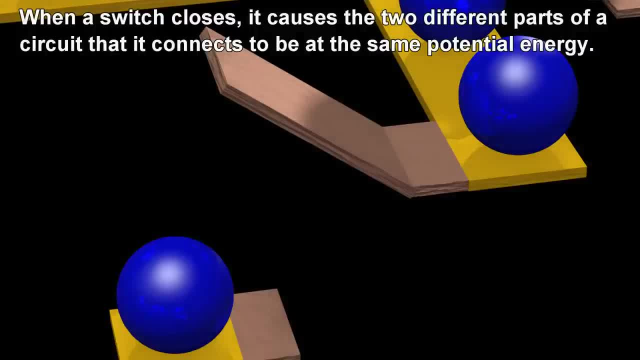 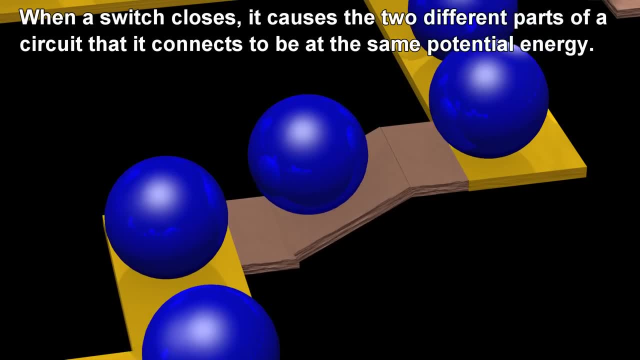 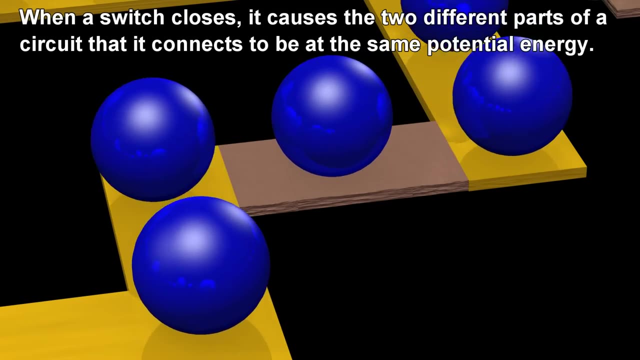 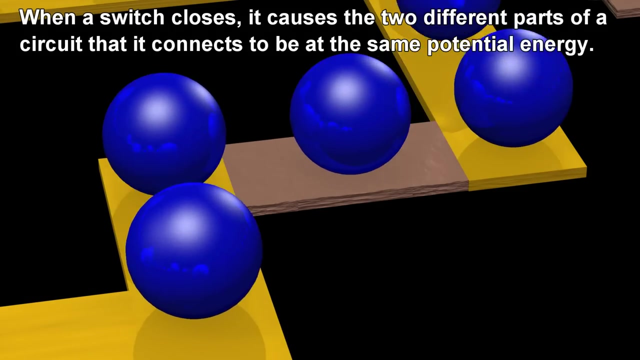 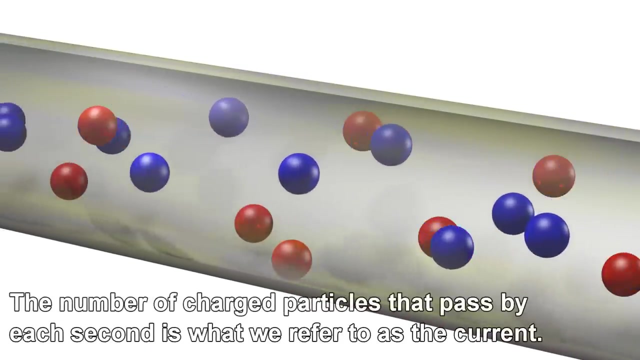 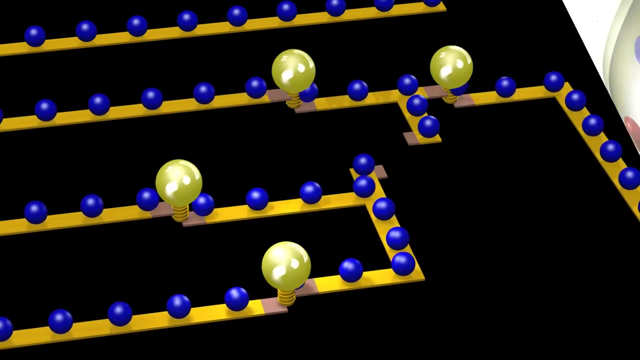 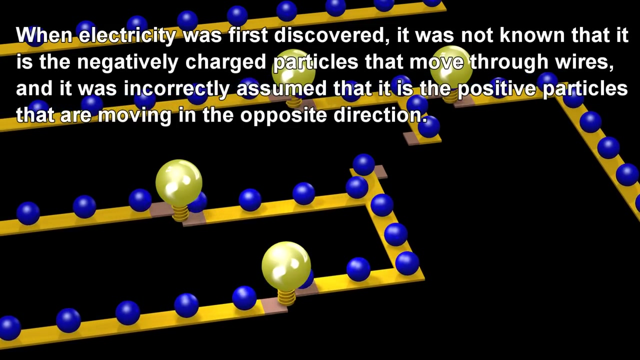 be at the same potential energy. The number of charged particles that pass by each second is what we refer to as the current. When electricity was first discovered, it was not known that it is the negatively charged particles that move through wires and it was incorrectly assumed that it's the positive.